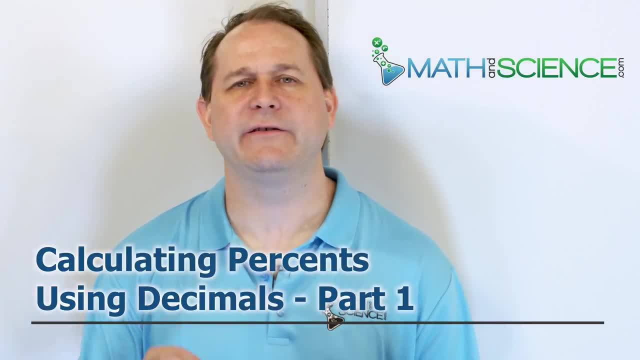 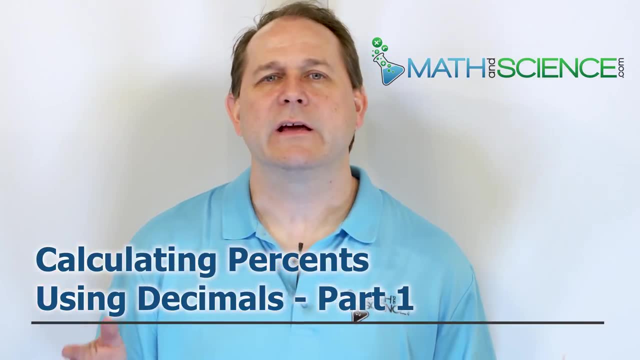 Hello, welcome back. The title here is called calculating percents using decimals. This is part one. So, if you remember, every percentage, every percentage that you'll ever see, can always be written firstly by a fraction that's equivalent to that percent, but also as a decimal equivalent. 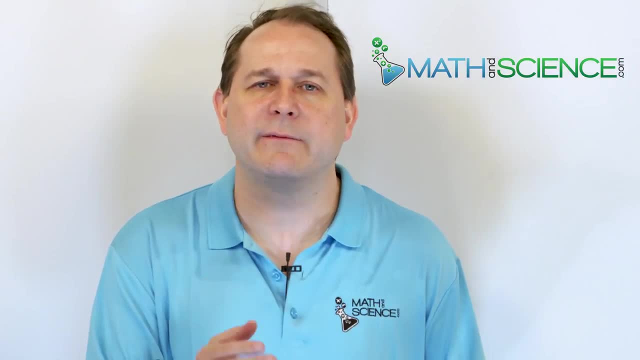 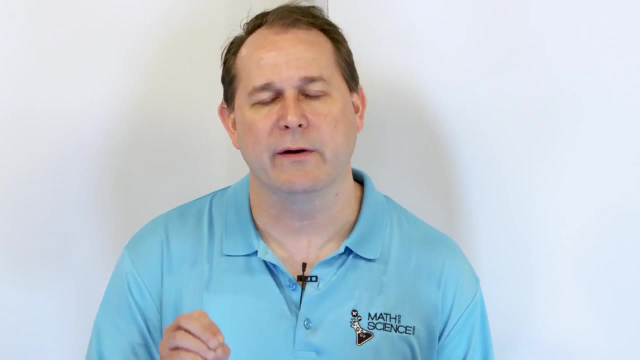 to that percent. In the last couple of lessons, we were calculating percents by multiplying by the fraction equivalent to get the answer. Here we're going to do the same thing, but we're going to be multiplying by the decimal equivalent of the percent in order to get the answer. 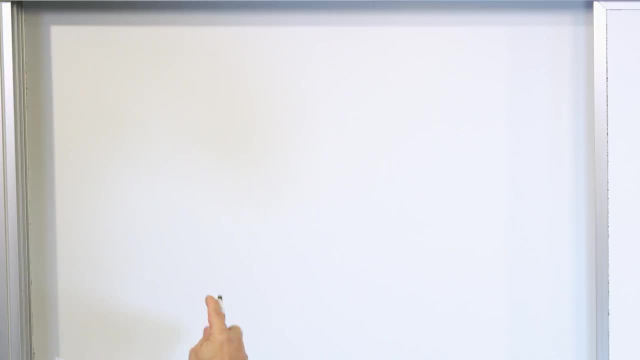 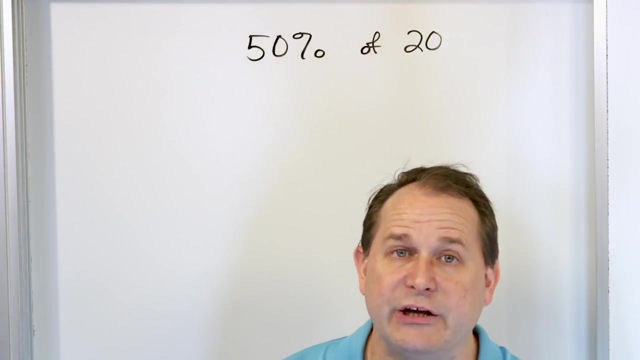 So it's going to be easier if we just explain with our first example. Let's say that we're trying to calculate 50% of 20 of something. So let's say that I have 20 pencils in my hand and I tell somebody I'm going to give you 50% of those pencils. What I'm telling you is since: 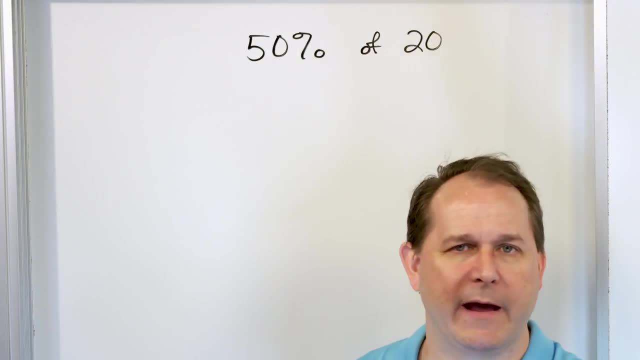 0% is nothing and 100% is everything of what I have, then 50% is right in the middle. So I'm going to give you 50% of what I have and I'm going to give you 50% of what I have. 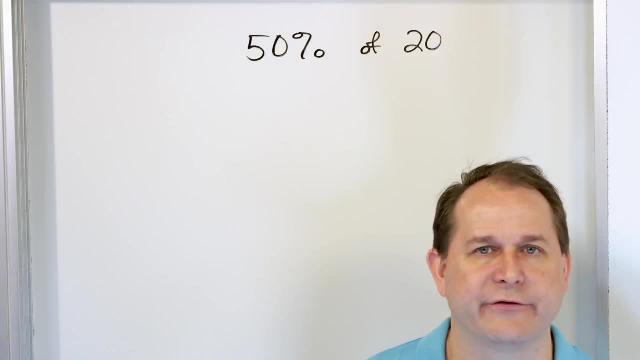 It is half of what I have. So you already know the answer to this problem. at the end of the day, If I give away 50% of this, I'm giving away half. I'm going to give you 10 pencils. That is a half. 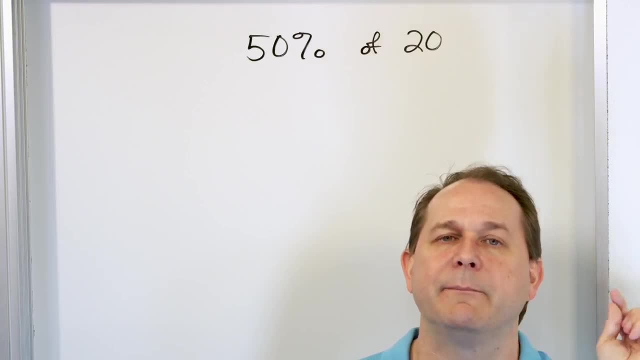 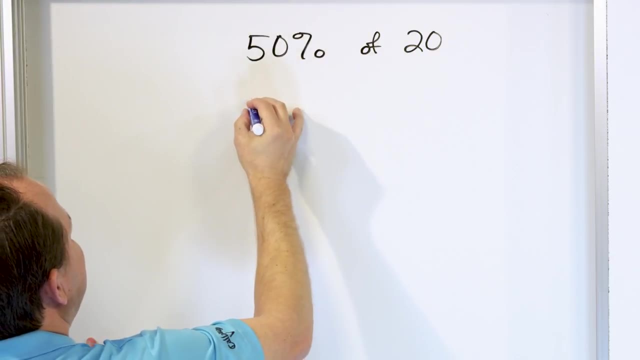 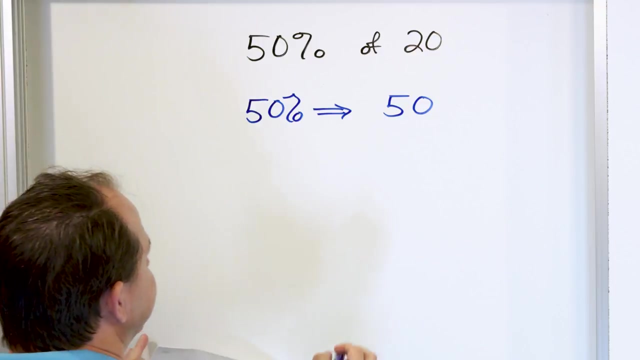 of 20.. But what we're going to do here is do it by multiplying by the decimal equivalent. Now, if I have 50%, then what I'm basically saying is that I'm going to take this 50% and I'm going to convert it by writing down the 50, and there's an invisible decimal after that. 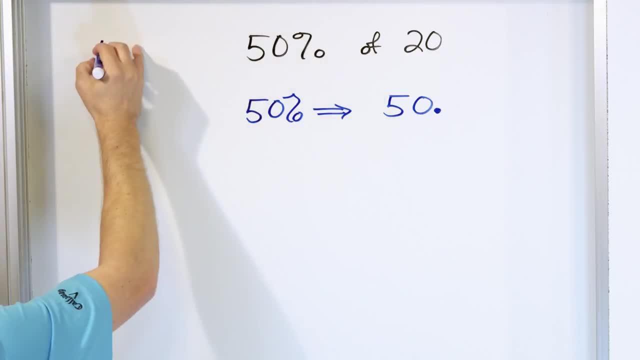 after the number 50. 50%, remember, 50% means 50 out of 100. That's what it means. So 50 divided by 100. When you divide by 100, what you're doing is you're taking the 50, and you're moving the. 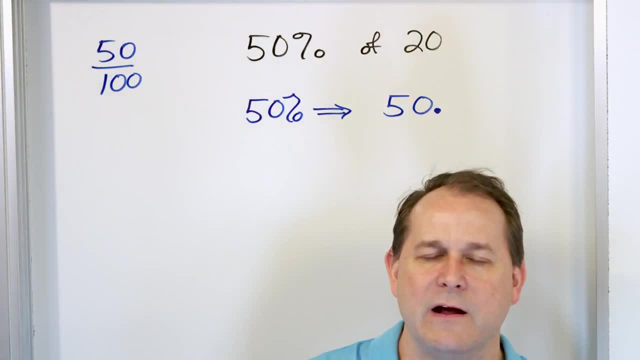 decimal two spots to the left. Remember, if you divide by 10, you move the decimal one spot to the left. If you divide by 100, you move it two spots to the left. Can you guess what would happen if you divide by 1,000? You'll move it three spots to the left. So here, 50% is 50 out of 100,. 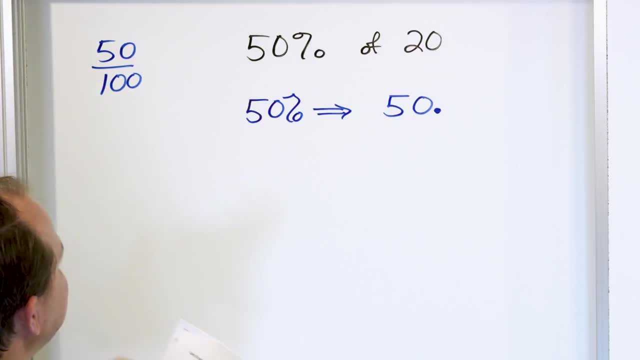 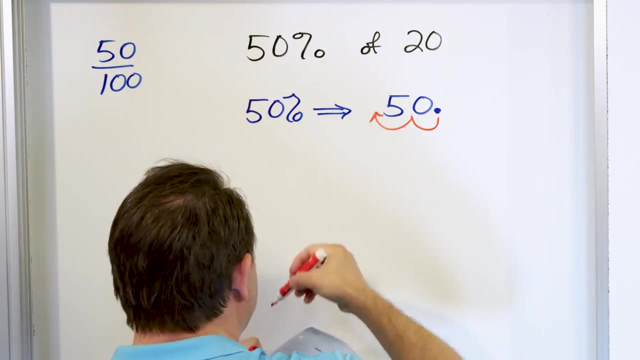 which means I take 50, and I divide. I divide by 100,, which just means that I take the decimal- here that is always at the end of the number, and I move it two spots to the left so it lands here. So what it basically is saying. 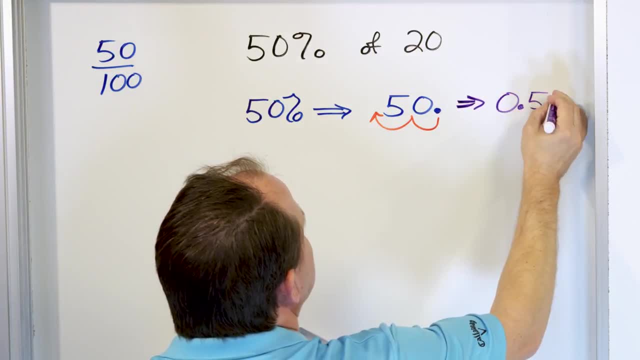 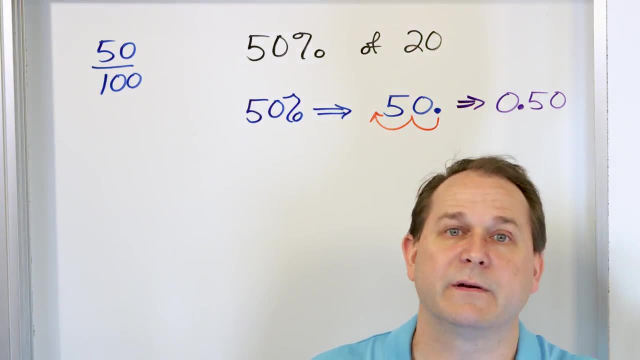 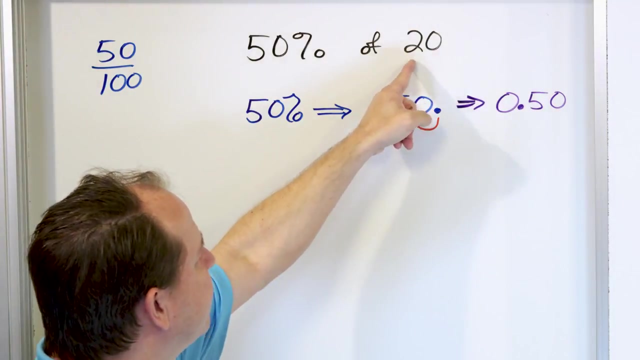 is that 0.50 is the decimal equivalent of 50%. So, just like in the last lesson, we found the fraction equivalent. We multiplied by the fraction to cut it down. right, Here we're going to be just multiplying by the decimal equivalent to cut it down as well. 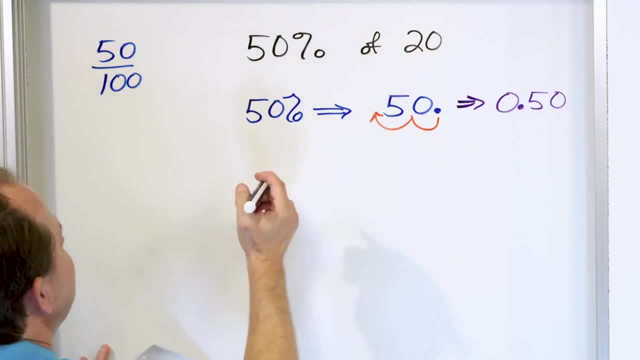 to cut the 20 down. So let's start off by saying we have, let's say, 20 pencils in a box and we're going to be taking 50% by multiplying by. I guess it'd probably be easier to say 0.5.. Notice that the answer I got. 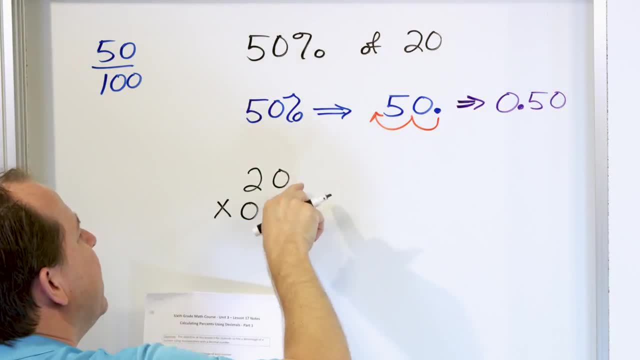 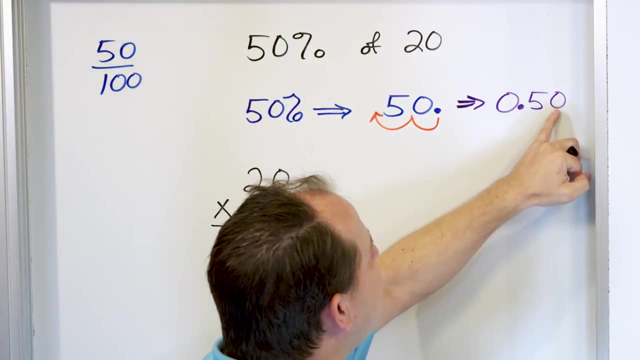 was 0.50.. I could put another zero there if I wanted to and then line it up differently, but it's just going to be easier to drop the last zero. When you have decimals here, the trailing zeros don't mean anything. 0.5 is the same as 0.50.. 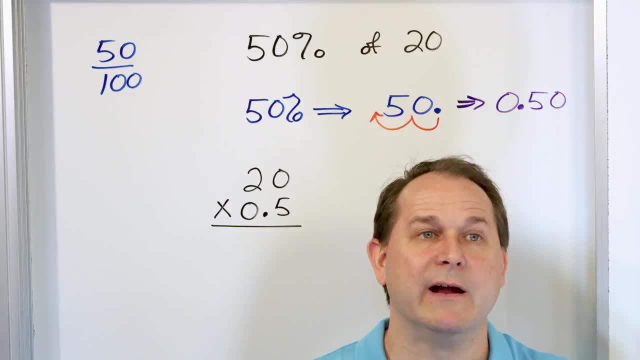 The same as 0.5, 0, 0, 0.. It's the same as 0.5, 0, 0, 0, 0, 0.. So it is 0.50, but the trailing zero. 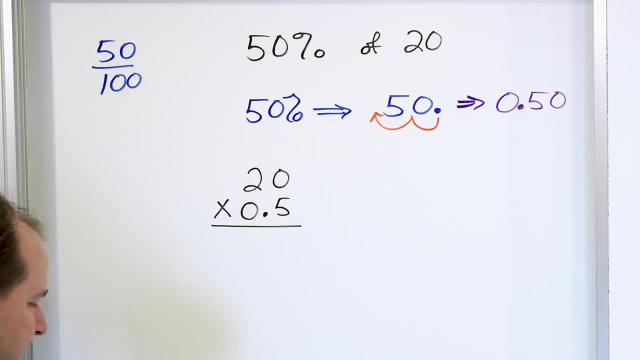 doesn't really matter. so I can just multiply by 0.5,. all right, And so what am I going to have? Ignore the decimal first of all. 5 times 0 is 0.. 5 times 2 is 10.. Drop a zero: 0 times 0 is 0.. 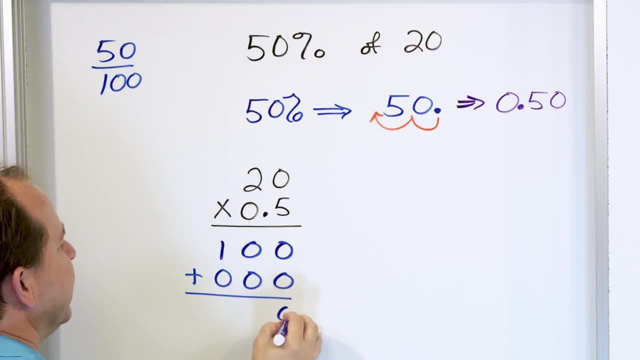 0 times 2 is 0, and I add: I'm going to have 0,, 0, 1.. So that's what I get, and now I have to figure out where do I put the decimal. So I'm going to have 0,, 0, 1.. So that's what I get, and now I have to figure out where do I put the decimal. 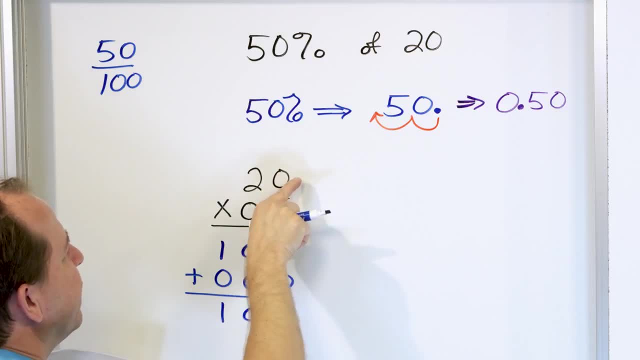 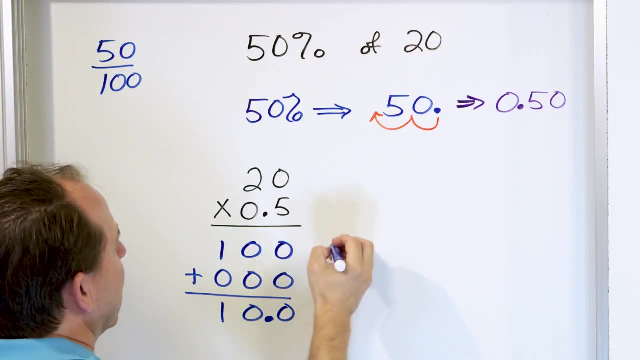 In my problem I only have one digit after the decimal. There are no digits after the decimal here, So I have to have the answer one digit after the decimal there: 10.0.. Another way of saying that is just 10,. 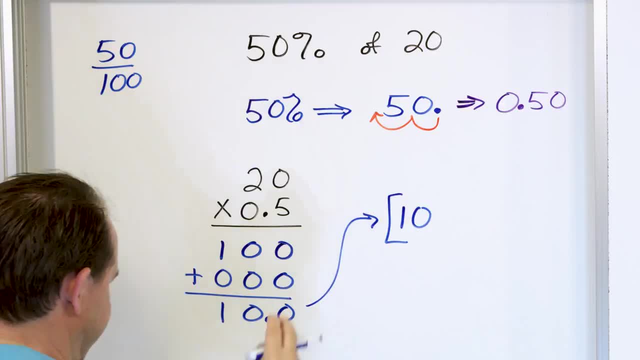 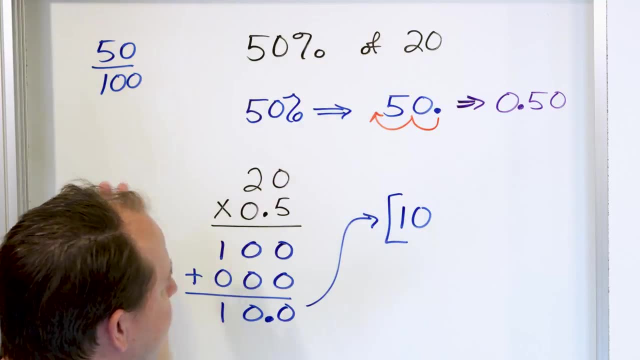 because 10.0 is exactly the same thing as 10.. So I'm just going to basically say it's exactly equal to 10, which is what we already said. 50% means half of whatever, and I'm taking half of 20, and so I know the answer is 10.. 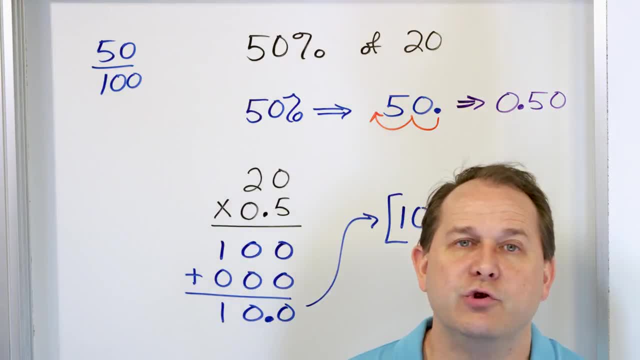 So you have freedom when you're working with percents. You now know that to calculate the percentage of something, you just can multiply by the decimal equivalent, and we know how to multiply decimals. So that's an application of multiplying decimals, right. 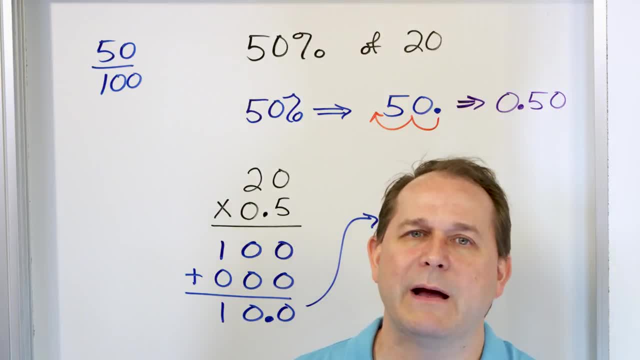 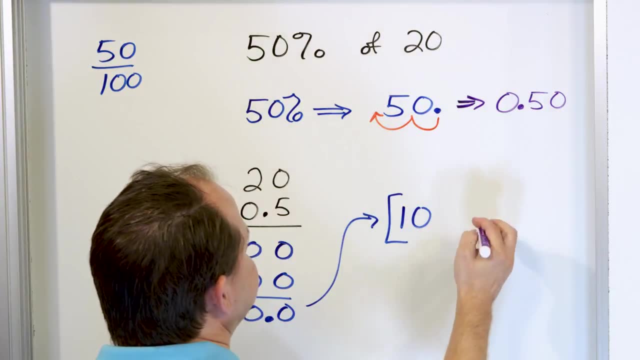 But we already learned in the last section that if you don't want to do this, you can just multiply by the fraction. In other words, I could multiply this times 1 half, because 20 times 1 half, what do you think that's going to come out to be? 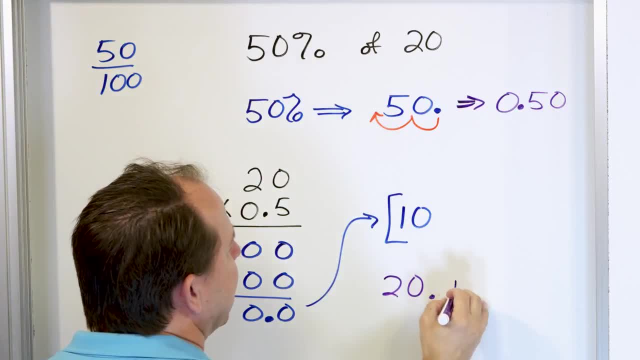 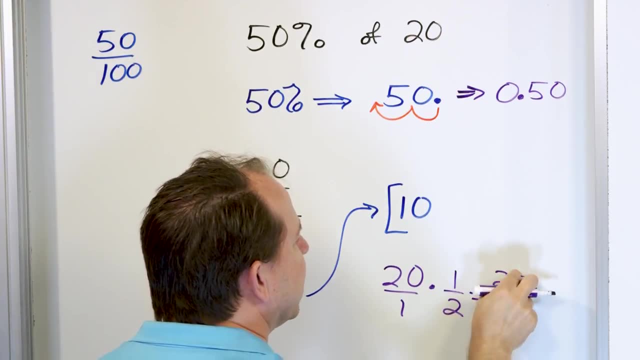 20, because 50% works out to be 1 half times 1, half right. 20 times 1 is 20.. 2 times 1 is 2.. And so then what I'm going to have is 20 divided by 2.. Again, it's 10.. 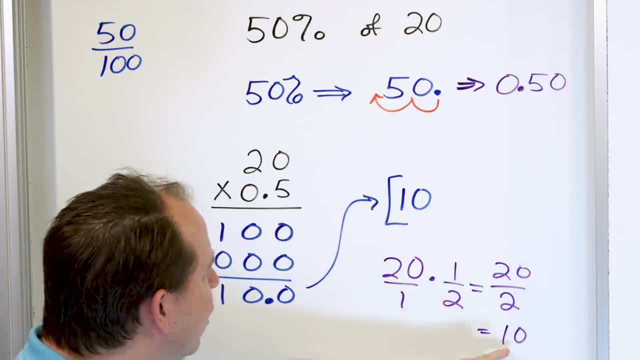 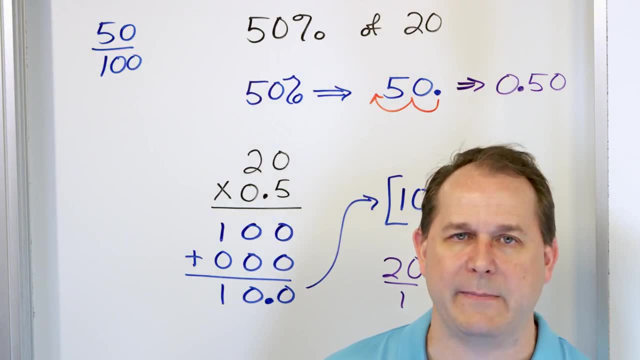 So whether I decide to multiply by the fraction equivalent and get an answer, or I multiply by the decimal equivalent and get the answer, the answers will be the same. So you have freedom in math Here. in these lessons, we'll be multiplying by the decimal equivalent. 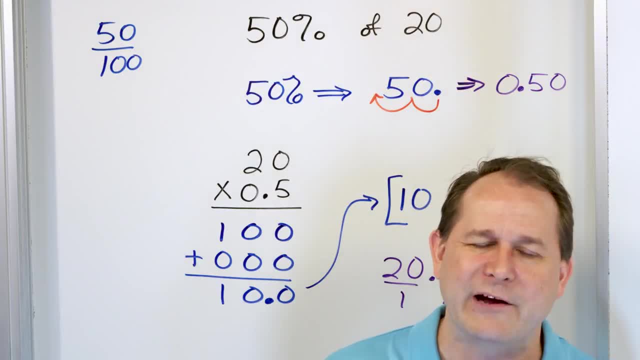 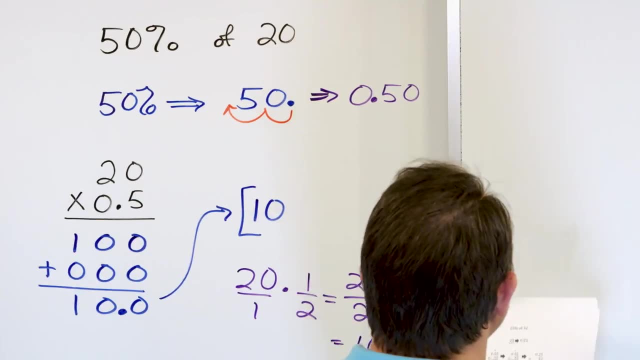 but just in the back of your mind, know that you could do it the other way with fractions if you want. You get the same answer. So, as always, first problem takes the longest. Let's crank through the rest of these guys. Let's calculate: What is 25?? 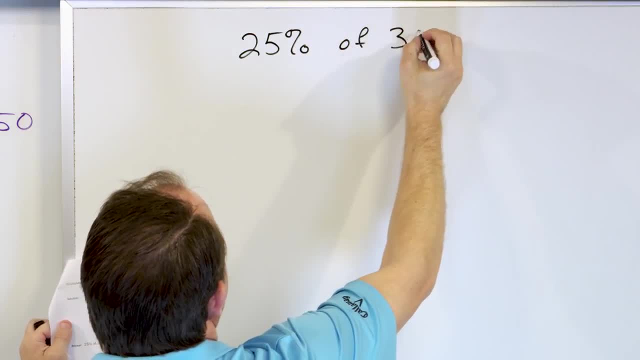 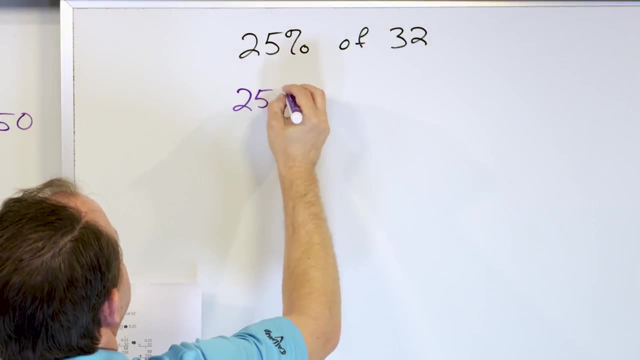 25% of 32.. Let's say I have 32 chickens and I'm going to give 25% of them away. First of all, 25%. what does that actually mean? Write the number 25 down. The decimal is here. 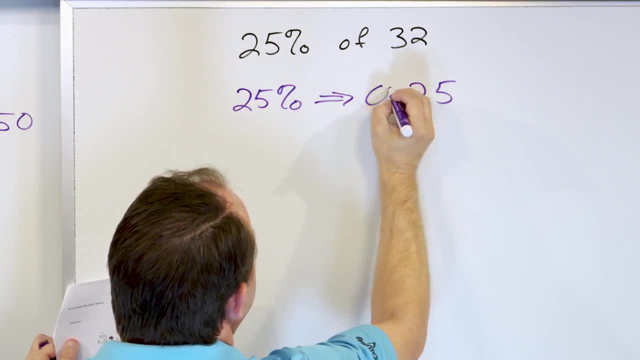 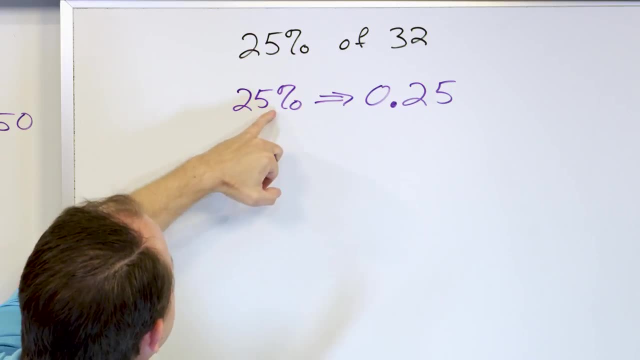 I'm going to move it two spots to the left, so it's going to be 0.25.. That's what 25% is. You take the decimal, move it two spots to the left, because it's 25 divided by 100.. 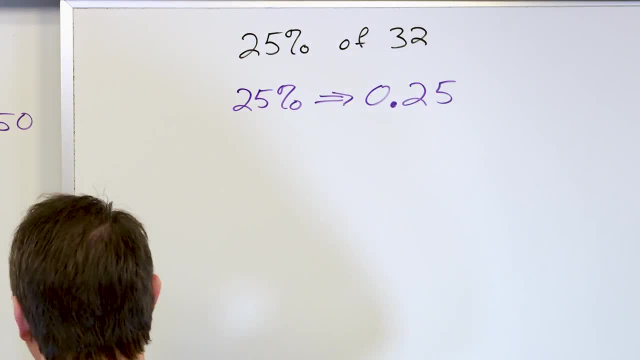 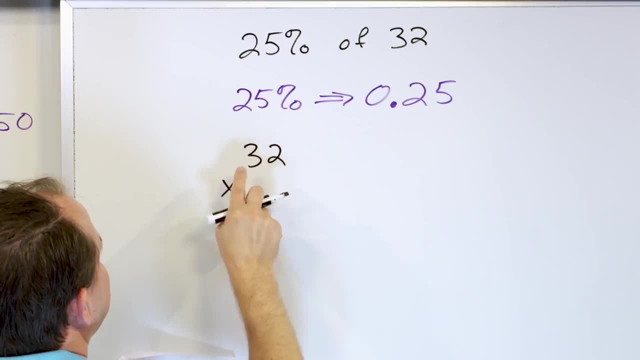 Two spots to the left, 0.25.. And so we're going to take the 32 chickens that we have and I'm going to multiply by. I guess I'll put it as 0.25 here, I'll write it as 0.25, and I'm going to multiply like this. 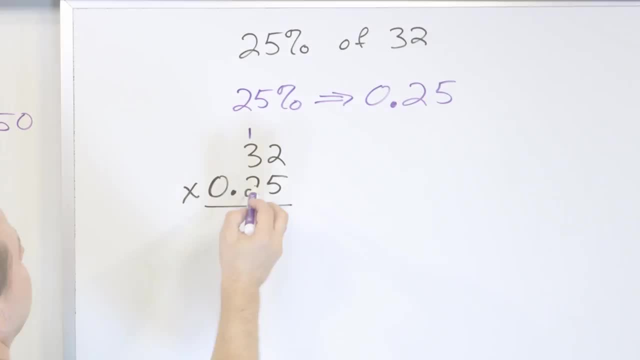 All right. 2 times 5, 10.. 3 times 5, 15.. One more 16,. so I'm just going to put the 1, 6 here. There's nothing else to carry to, so I don't have to do anything there. 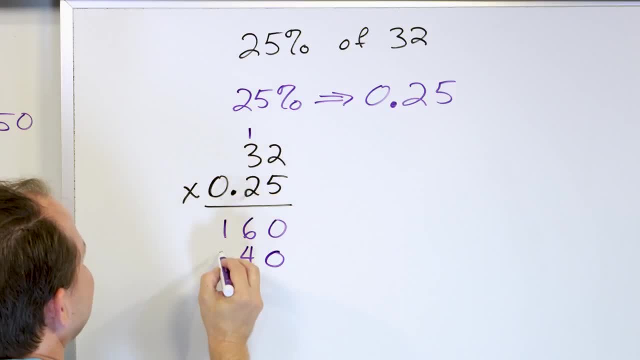 Drop a 0 here. 2 times 2 is 4.. 2 times 3 is 6. And I guess you have 0.. 0 times this and 0 times this is basically going to do nothing. I guess I could just go ahead and put 0.. 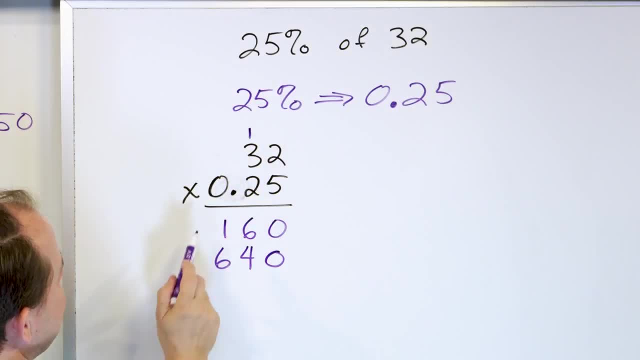 So I have: the 2 times 2 is 4, and the 2 times 3 is 6.. And now technically you have to multiply by the 0, so you would drop two 0s here, But the 0 times 2 would be 0, and the 0 times 3 would be 0. 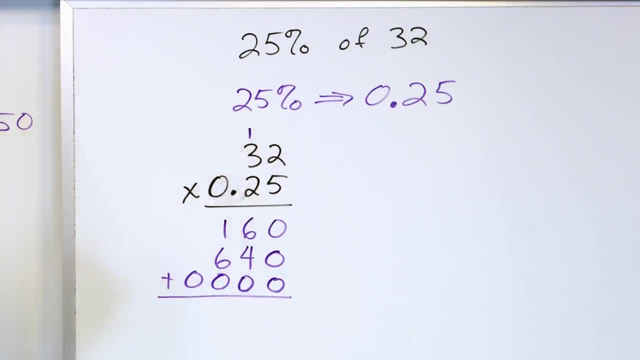 So really, if you have 0, point something, there's no reason to multiply by the leading 0. You see it does nothing. All of these things up, These 0s give you 0.. 6 and 4 give you 10.. 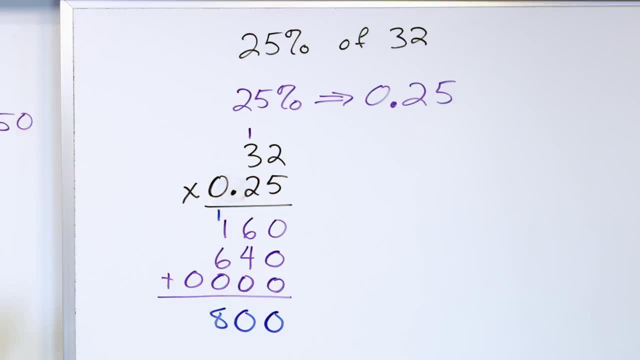 And then 6,, 7,, 8.. And then you have a 0 right there. Where does your decimal go? We have two positions after the decimal in the entire problem, so I must have two positions after the decimal in my problem. 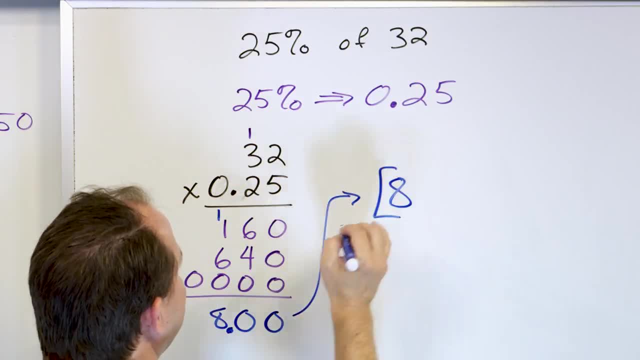 And 8.00 is exactly the same thing as 8, so I'm going to write it as 8 there. So if I had 32 chickens and I'm going to give away 25% of them, then I'm giving away 8 chickens. 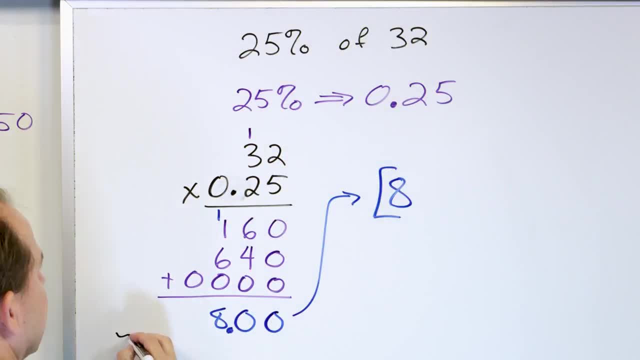 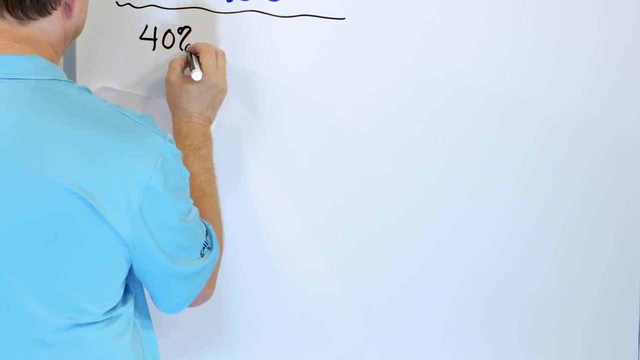 That's basically what that means. All right, So let's take a look at the next problem. Let's calculate 40% of 25.. So a little bit less than half, because 50% will be half of this, and this is a little. 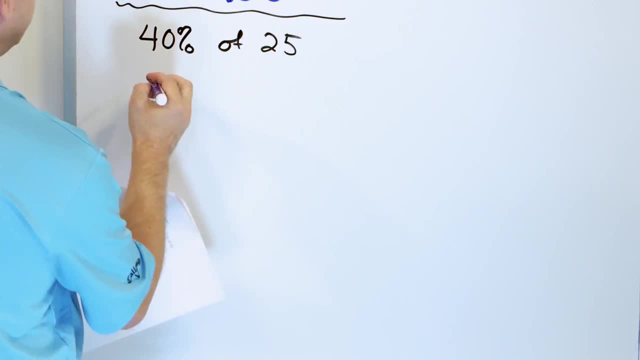 bit less than half of 25.. So first of all, you need to recognize that 40% is going to be equal to 0.40.. Why? Because if I take 40 and have a decimal at the end and move it one, two positions to, 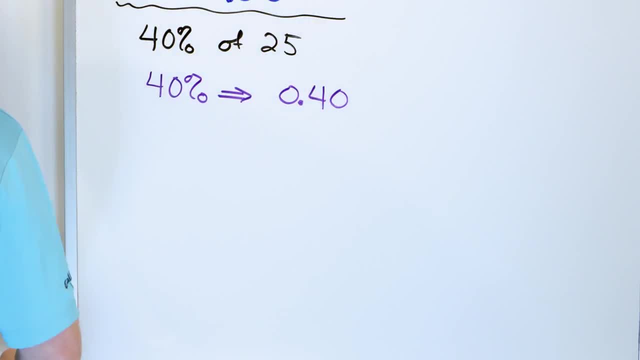 the left, It'll be 0.40.. So I'm going to multiply the 25 times this decimal: 25 times 0.40.. I'll just write it as 0.4.. You don't need the trailing zero. 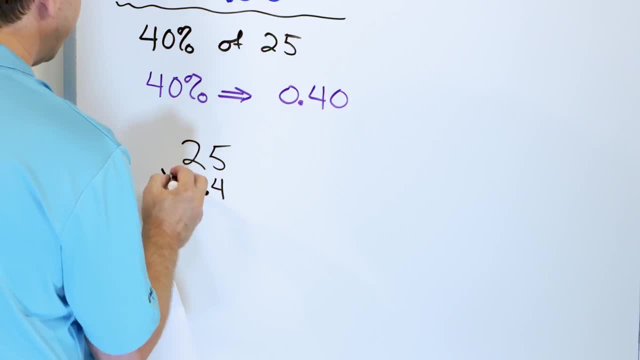 It's not going to do anything, So just write it as 0.4 there, And then we're going to multiply, All right. Next, what are we going to have? Five times four? Let's change colors here. Five times four is 20.. 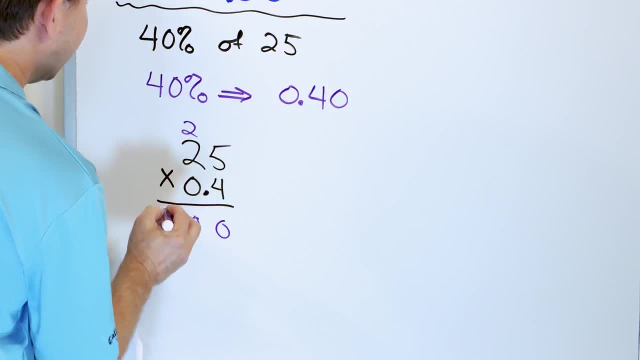 Carry the two Two times four is 8,, 9,, 10.. So there's your 10.. Now we're multiplying by a zero there, So we don't need to, But I'll show you one more time. You drop a zero. 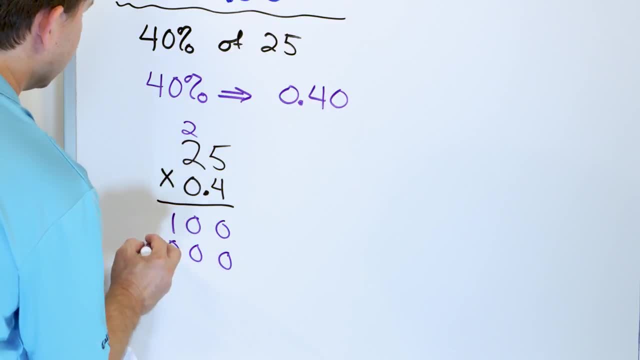 Then zero times five is zero. Zero times two is again zero. And what are you going to have? One zero, zero. That's what you're going to have. And then where does your decimal go? There's one position after the decimal in the entire problem statement. 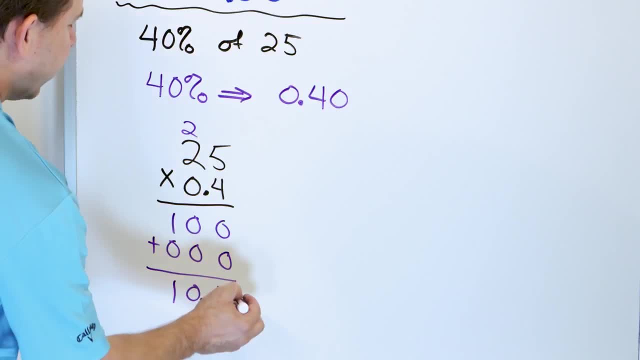 So I have one position after the decimal in my answer, And 10.0 is the same thing as 10.. That's the final answer. So if I take 40% of 25, it's going to be a little bit less than half. 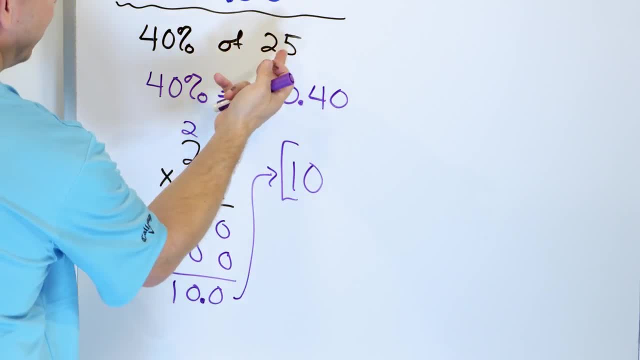 And so that's because half of this would be 12.5, 12 and a half, so a little bit less than that is 10.. 10 is the final answer, So 40% of 25 is 10.. That's what that basically means. 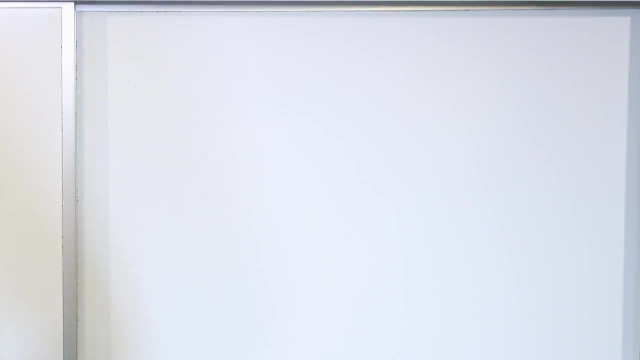 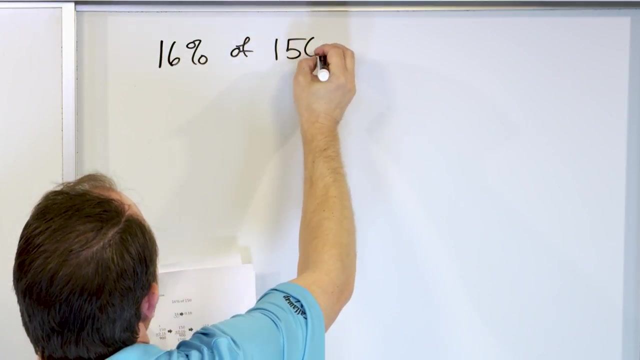 All right, Let's take a look at problem number four. Let's calculate 16% of 150.. 16% of 150.. First thing to recognize is that when you actually have 16%, that's exactly what you're doing. 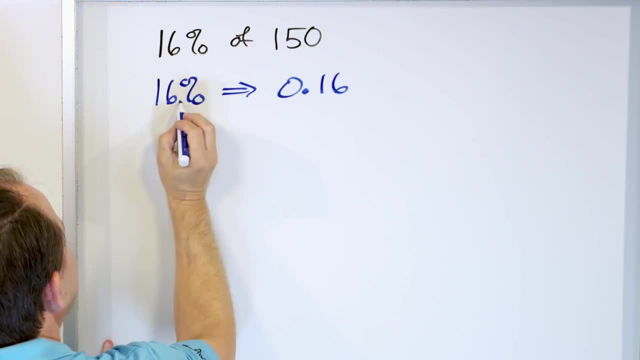 It's exactly the same thing as 0.16.. How do you know? Because if you start with a decimal here and move it two spots to the left, 0.16 is what you get. All right, So let's calculate the number 150, and we're going to then multiply by zero. 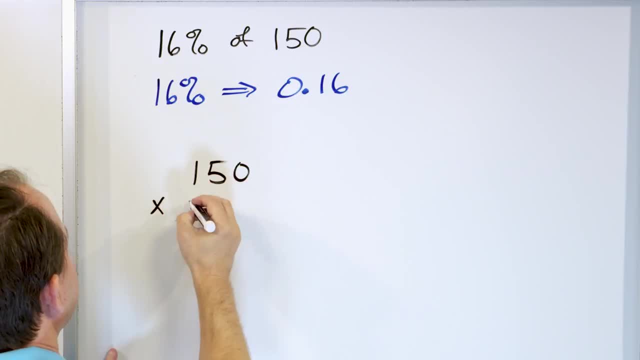 Let's do it as sorry, let me erase the zero. I should line my numbers up a little better: 0.16.. And you completely ignore the decimal point. remember when you multiply decimals until the end. So let's say 6 times 0 is 0.. 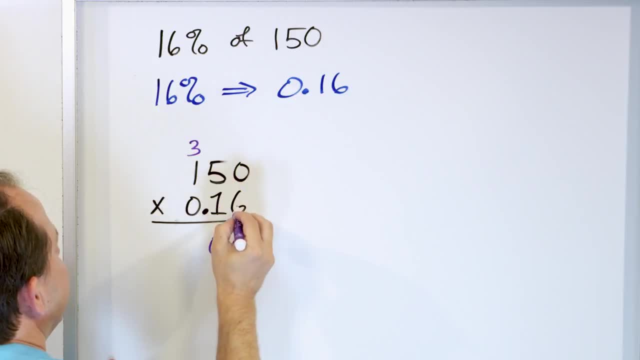 6 times 5 is 30.. Carry the 3.. 6 times 1 is 6.. 7,, 8, 9 goes here. Now we have to drop a zero. 1 times 0 is 0.. 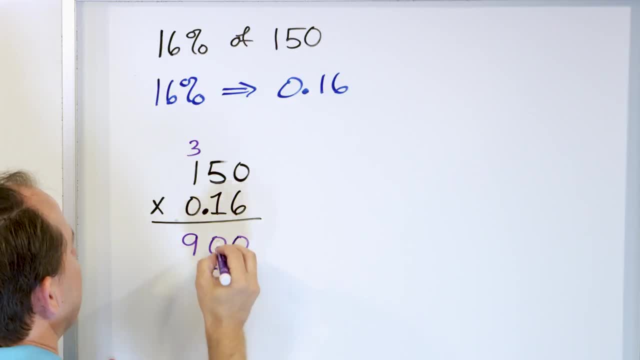 1 times 5 is 5.. 1 times 1 is 1.. Now we could multiply by that leading zero, but we're going to drop zeroes and then everything multiplied is going to give you all zeroes. It's not going to do anything. 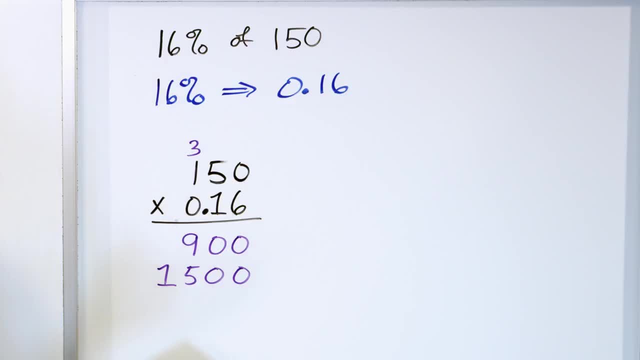 So we're going to just stop there And we're going to add everything up. We have a zero here, a zero here, 9 and 5 is 14.. And then we get a 2 right here, And then we're just going to stop there. 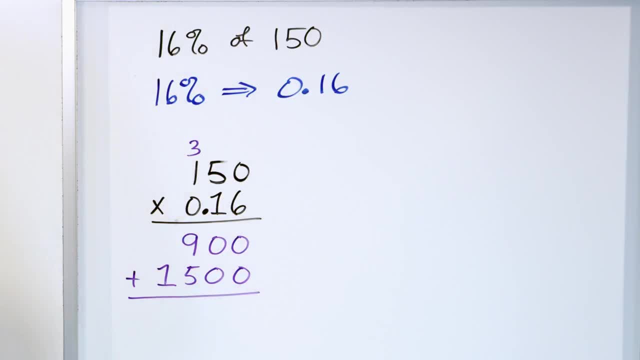 And we're going to add everything up. We have a zero here, a zero here, 9 and 5 is 14.. And then we get a 2 right here, And then where does the decimal go? We have two positions after the decimal in our entire problem. 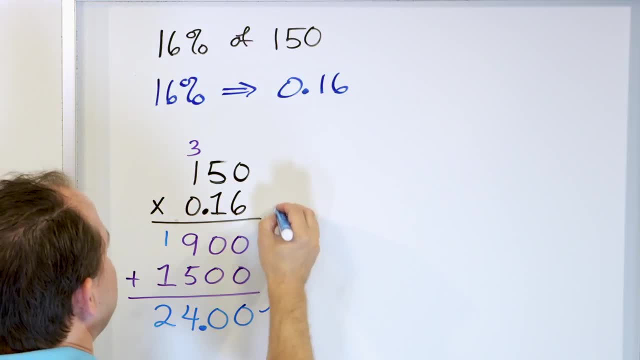 So that means we have to have two positions after the decimal in our answer, And so the answer is 24.. So if I have $150 and I plan to give 16% away to my mother, I'm giving her $24.. That's what that means. 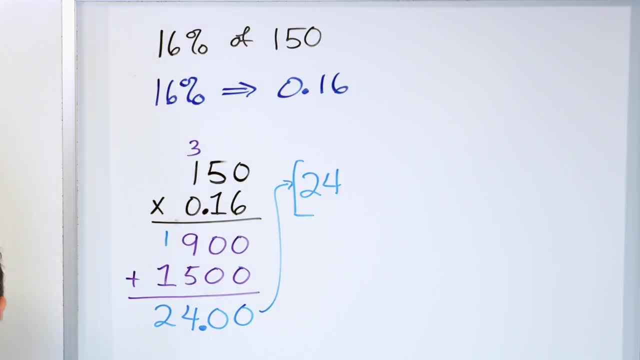 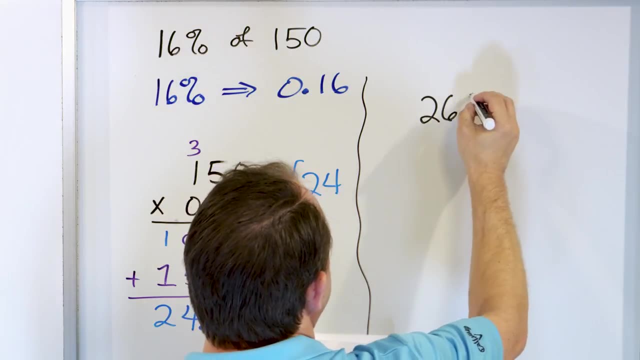 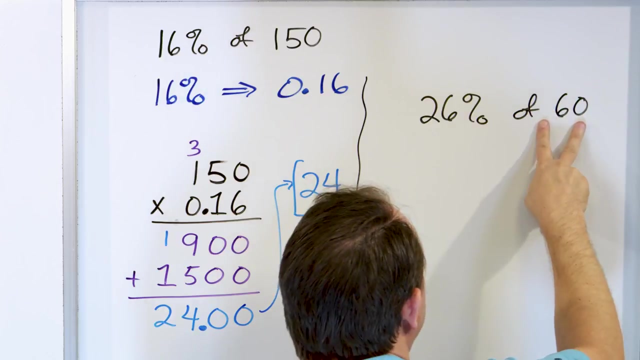 So 16% of 150 is equal to 24.. All right, Let's move along. Let's say we're going to calculate 26% of 60.. 26% of 60. Remember, 25% would be exactly one quarter of this. So it's going to be a little bit more than one quarter. 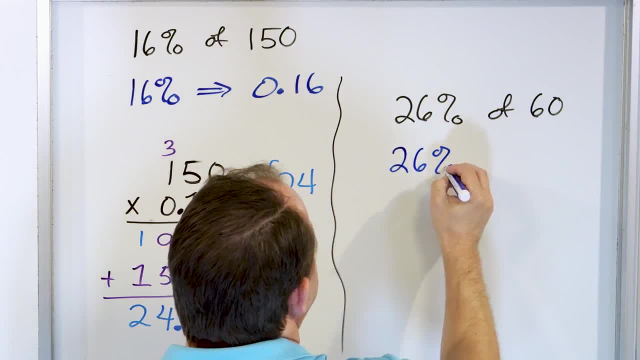 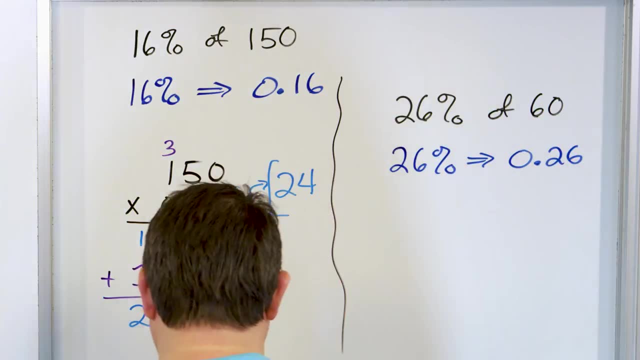 The first thing to remember is that 26% is 0.26. Because if you have a decimal at the end, you move it two spots to the left. it's 0.26.. So now we multiply, We take the 60,. 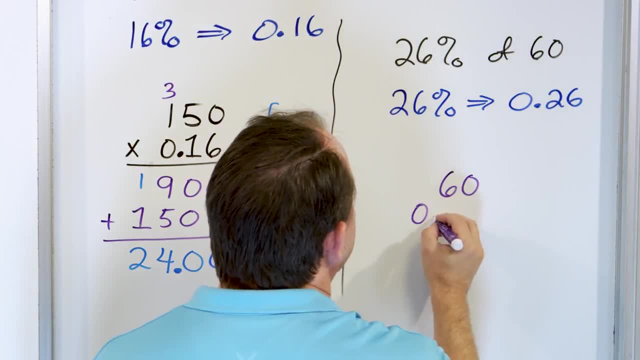 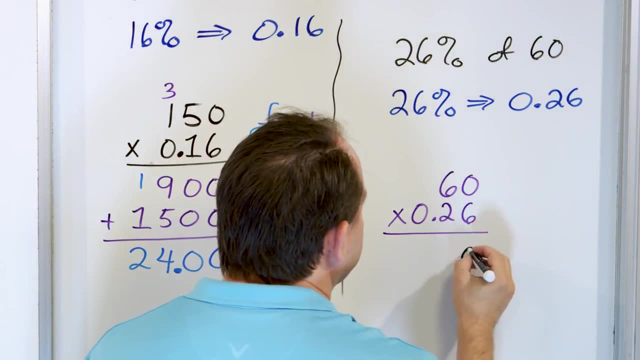 and we multiply by the percentage, but as a decimal: 0.26.. Multiply Like this: 6 times 0 is 0.. 6 times 6 is 36.. So you carry the 3, but there's nothing there. 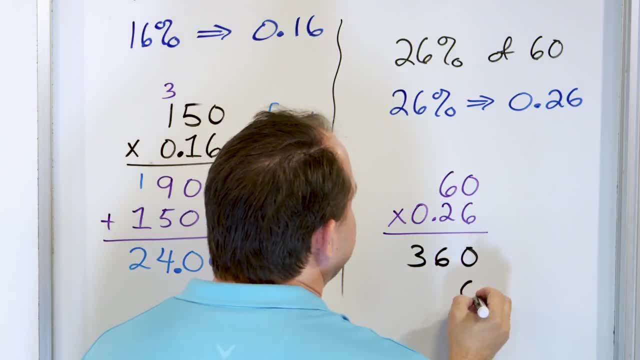 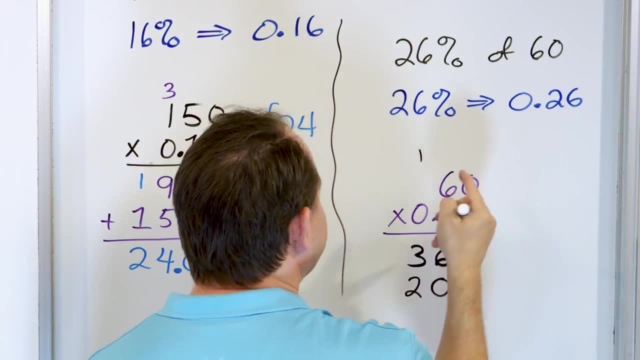 so just drop it down there. And now we multiply by the 2, so we drop a 0.. 2 times 0 is 0, and 2 times 6 is 0.. is 12.. We're going to carry the one here. Actually, there's nothing to carry to, so we just put the 12. 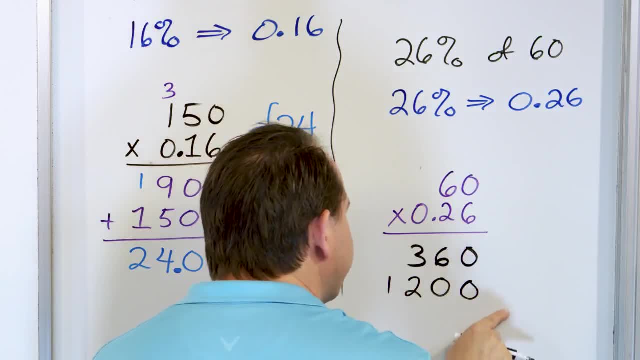 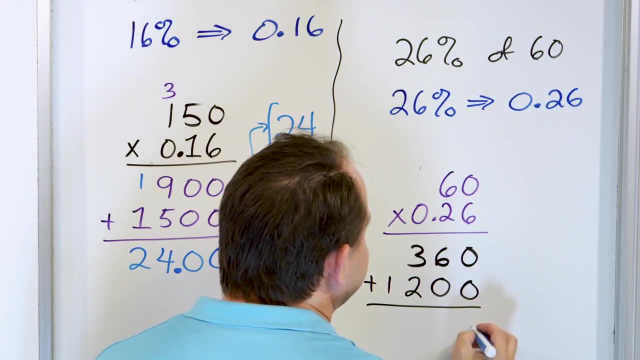 down here, And then now we need to multiply by a leading zero. but that's just going to add zeros everywhere, so it's not going to really do anything. So we're going to drag it down like this: Zero plus zero is zero. then this is going to give you a six and this is going to give you. 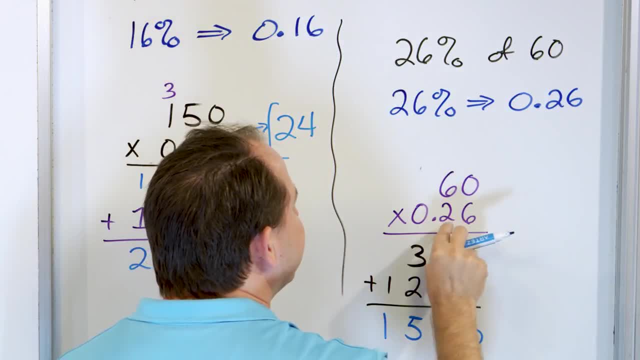 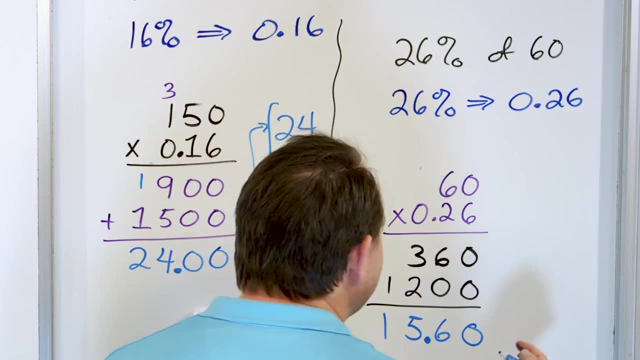 a five and this is going to give you a one. And in our problem there are two positions after the decimal in our entire problem, so the decimal point has to come right here. So the answer is 15.60, or you could write it as 15.6, because, remember, trailing zeros don't really add much. 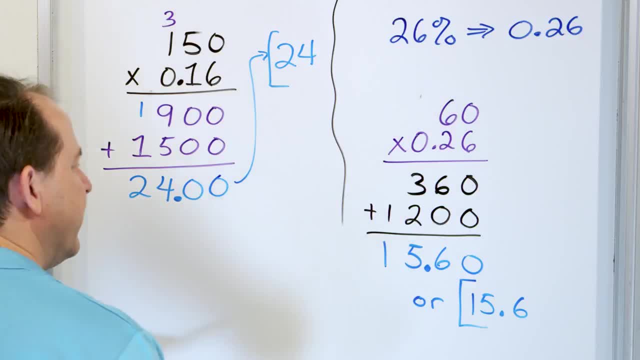 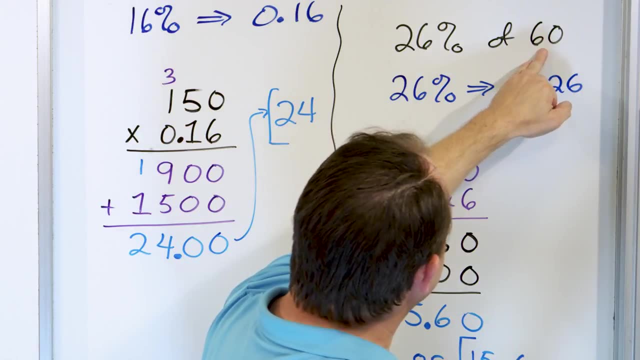 meaning in terms of decimals, 15.6 is the same thing as 15.60.. So if I have 60 buffalo- or that's probably not a good example- if I have 60 pizzas, let's say, and I'm going to give away- 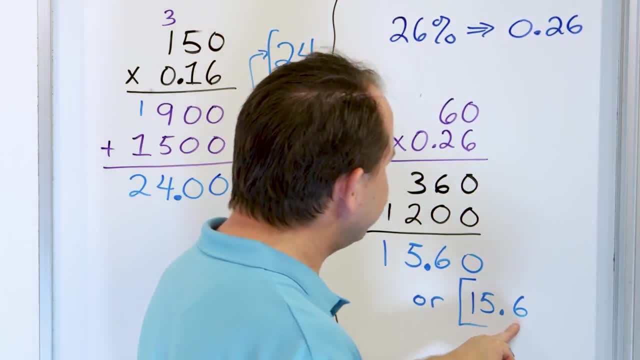 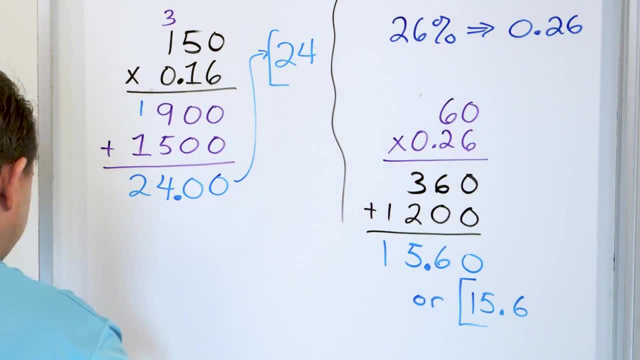 26%, then I'm going to give 15.6 pizzas away, which means 15 pizzas plus a little more than half of another pizza. That's basically what that means. All right, I don't want to cut any buffaloes in half. 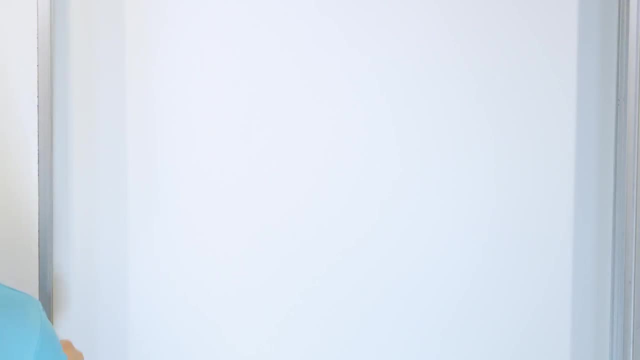 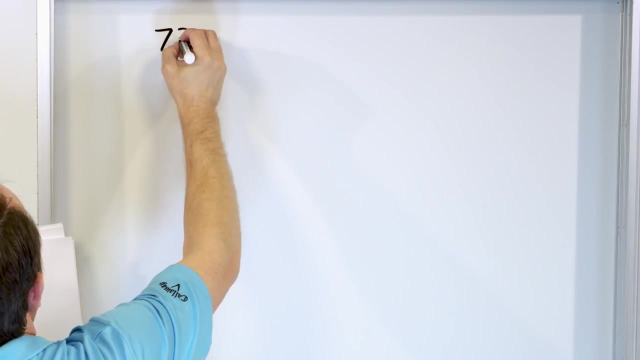 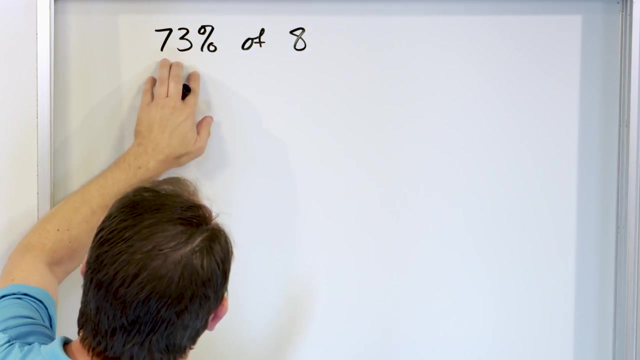 so that's why we changed it to pizza. I think we only have a couple more problems. Really, this is an exercise in multiplying by decimals. essentially, Let's calculate 73% of eight. 73% of eight, So 50% would be half of that. This is quite a bit more than half. 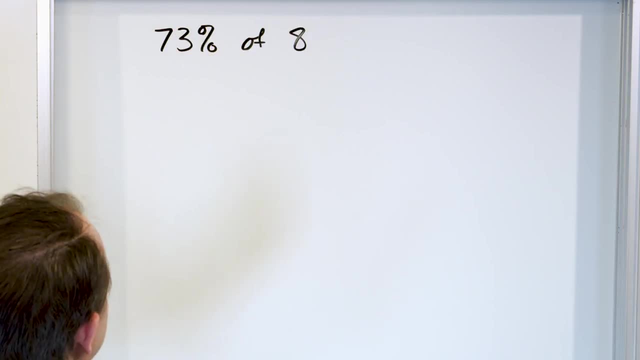 so we know it's going to be bigger than four. You can kind of estimate the answer: It's going to be around five or six, Something like that. I'm not totally sure, Maybe around seven even. Let's go ahead and calculate. 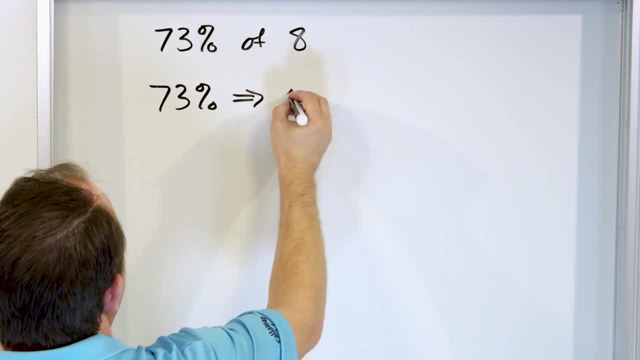 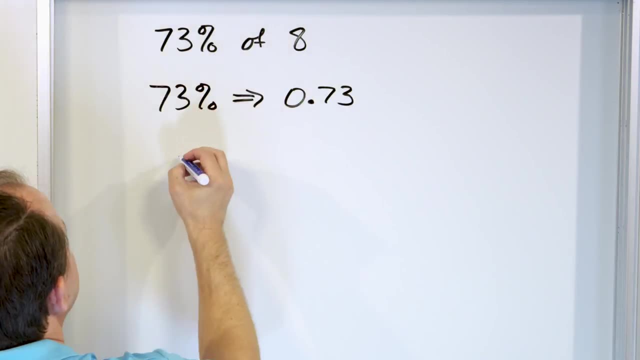 it. 73% is, as a decimal, 0.73, because if you move the decimal two spots to the left, that's what you get. Now we're going to take 0.73, and we're going to multiply by eight. So when you 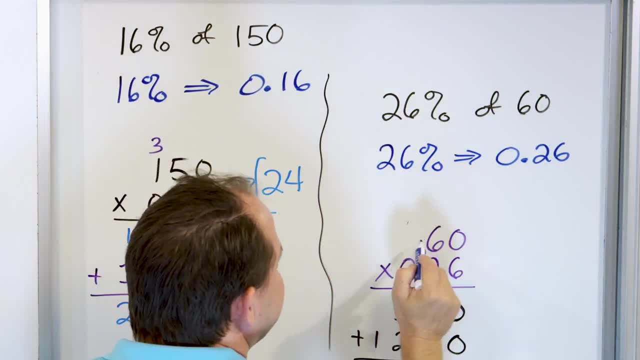 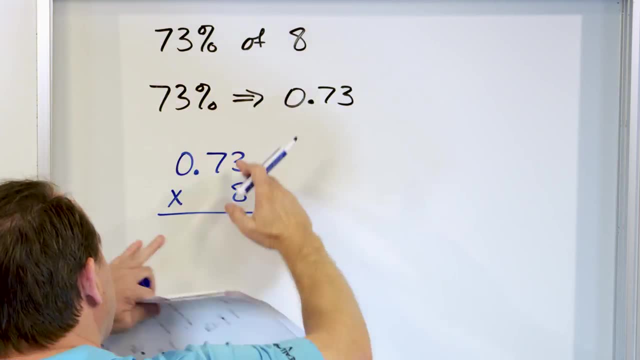 multiply. notice. in the previous problems I did 60, the whole number times the decimal and you can get the correct answers Here. I'm going to take the decimal and multiply it by the eight. So if you're reversing the order of the multiplication, it doesn't matter, You can. 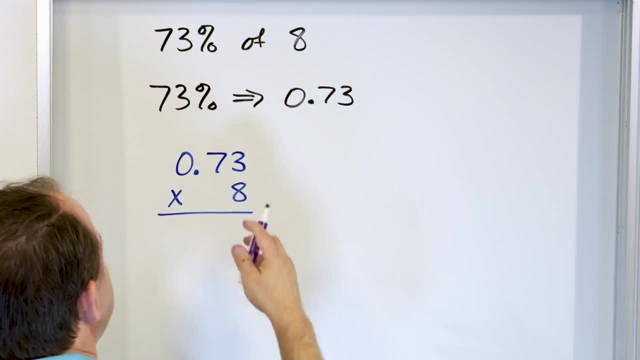 multiply it whatever way you want, You get the same answer: Eight times three, 24.. Eight times seven, 56.. 57,, 58. Carry the five And then eight times zero is eight. I'm sorry, eight times zero. 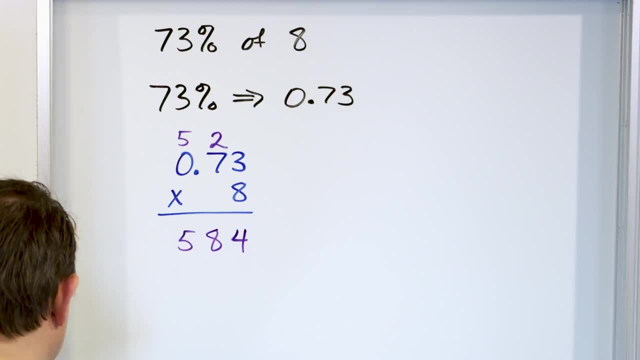 is zero, and then you have the five more, So you have 584.. Where does the decimal go? We have two positions after the decimal in our problem, so we have to have two positions after the decimal here: 5.84.. 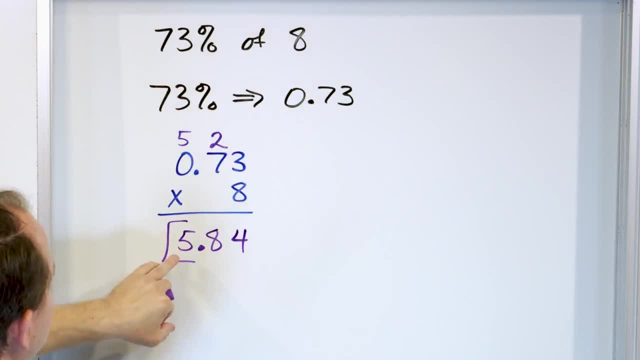 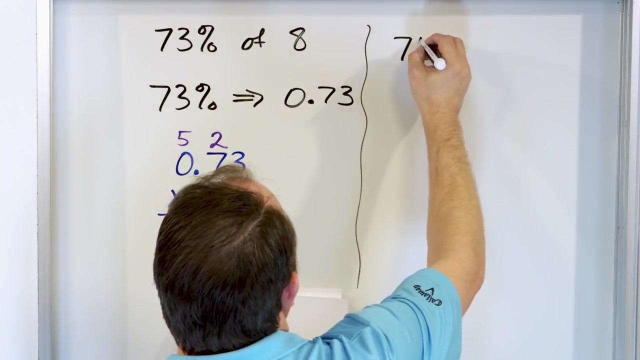 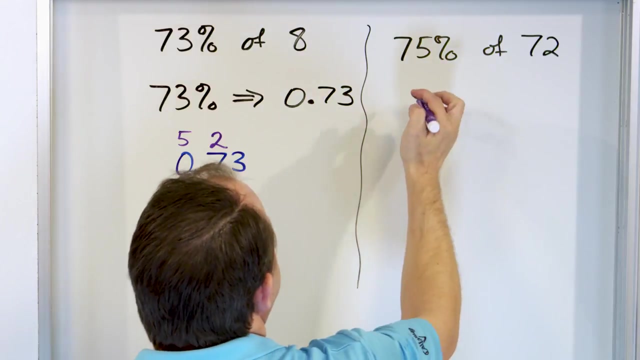 So if you told them that we would give them 73% of my pizzas, then it would be more than five pizzas, but less than six. It would be 5.84 pizzas. That's what that boils down to. All right, Let's move along to 75% of 72.. Now, first of all, what is 75%? It's very easy to. 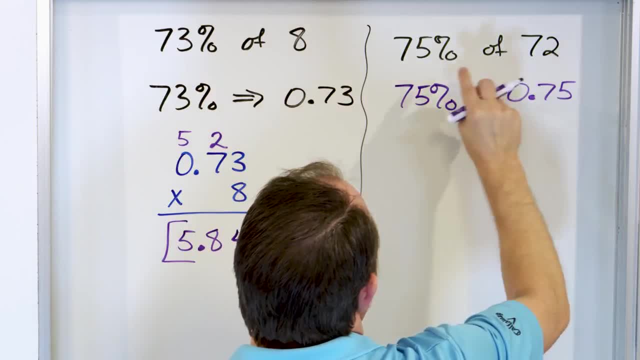 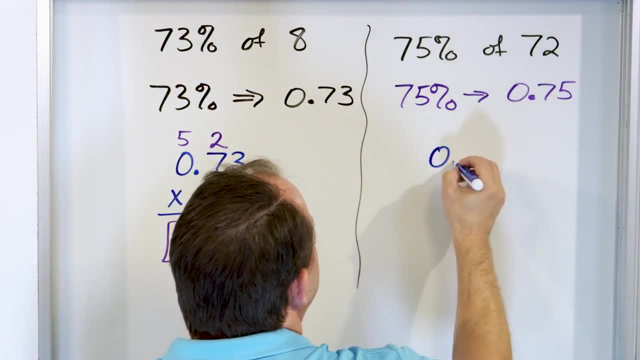 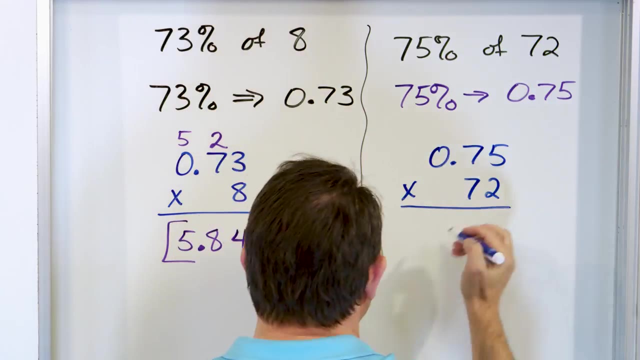 make a decimal, 0.75.. If you just move it two spots to the left, 0.75.. Now we can take and multiply these numbers together: 0.75 times 72.. Whoops, I already put a multiplication symbol there, And then we just go. 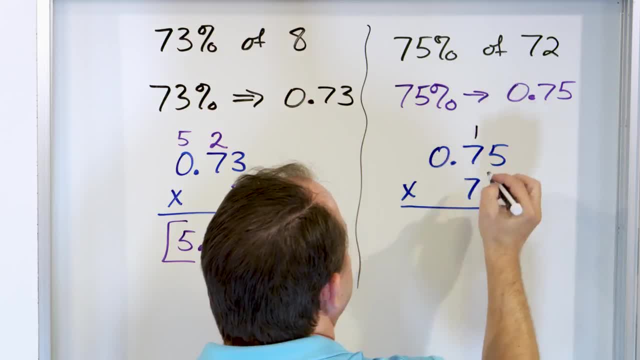 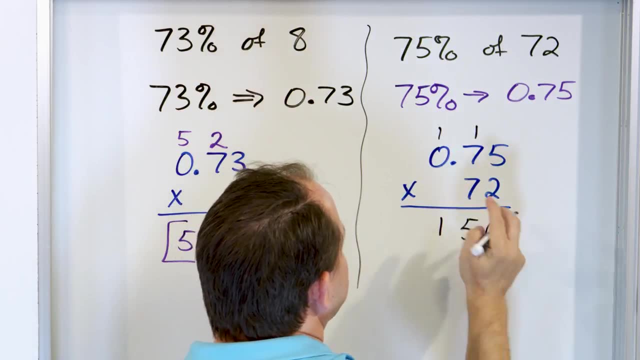 down here and just crank through it: Five times two, 10.. Seven times two, 14.. One more 15.. And then two times zero: zero. One more is one. Now we have to multiply by this drop a zero Seven. 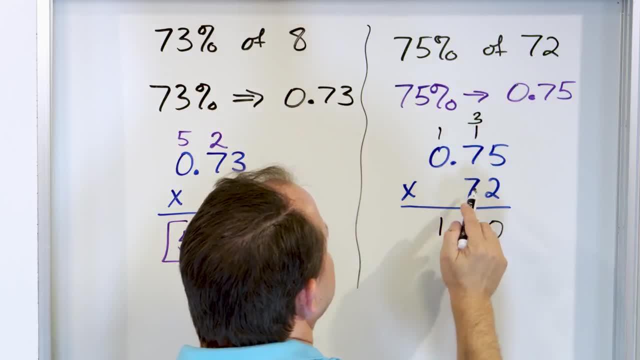 times five, 35.. Carry the three, Seven times seven, 49.. Then up here, 50,, 51,, 52.. Carry the five And then seven times zero is zero, And then five more is five, And then we add all of these together, All right. 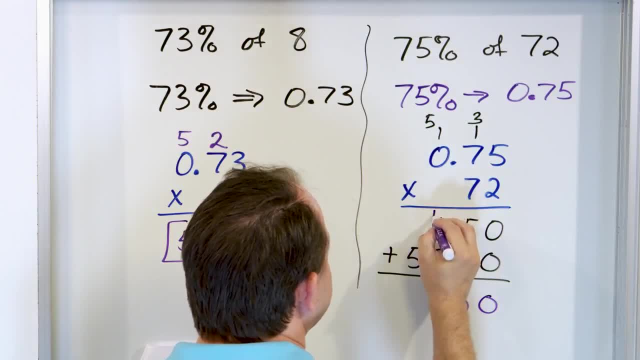 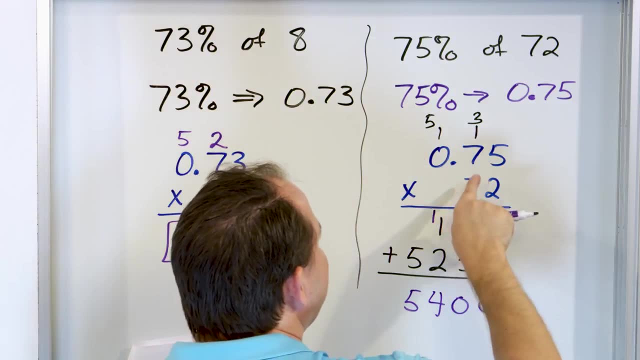 So we have zero plus zero. zero, Five plus five is 10.. Carry that: one, two, three, four And then the five drops down. So we have five, four, zero, zero. And look at our problem: We have two. 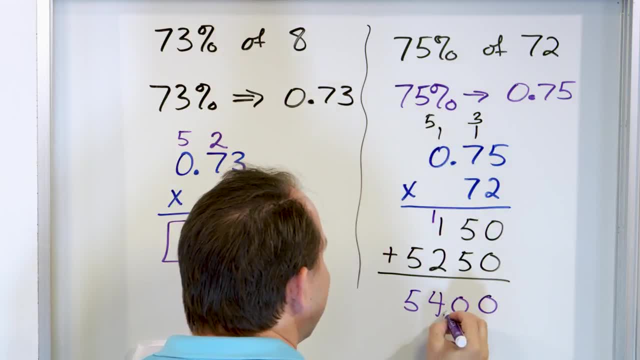 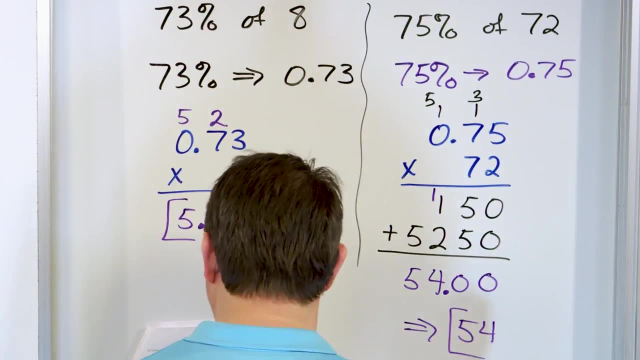 positions after the decimal in our whole problem. So that means we have to multiply by two, We have to have five, four point zero, zero, which just means a number of exactly equal to 54. That's just a whole number of 54. So if I had 72 potatoes and I was going to give 75% of them, 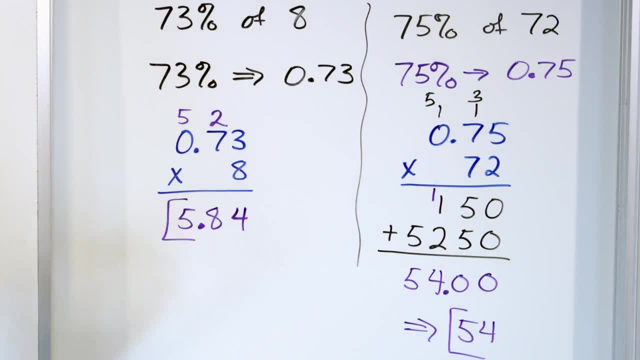 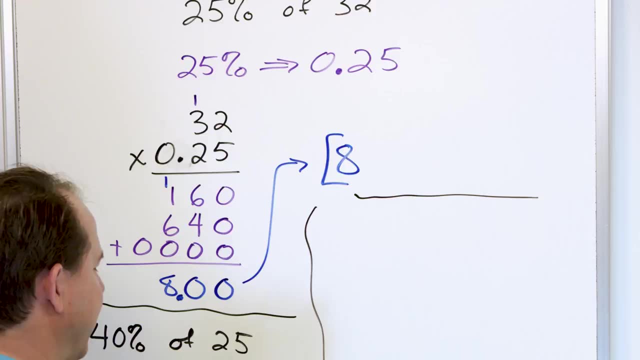 away. I would be giving away 54 potatoes. That's basically what that means. All right, Here is our very last problem in this lesson, So let's take a look at the following: What about 90% of 37? 90%. 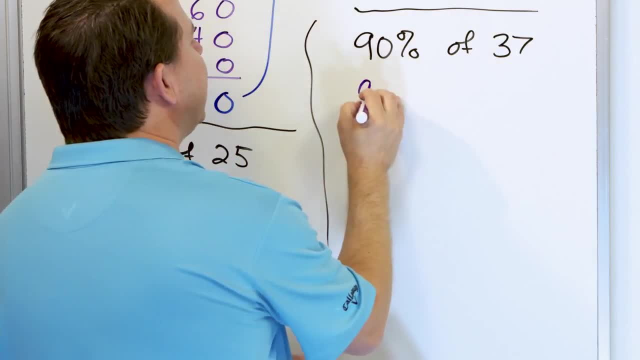 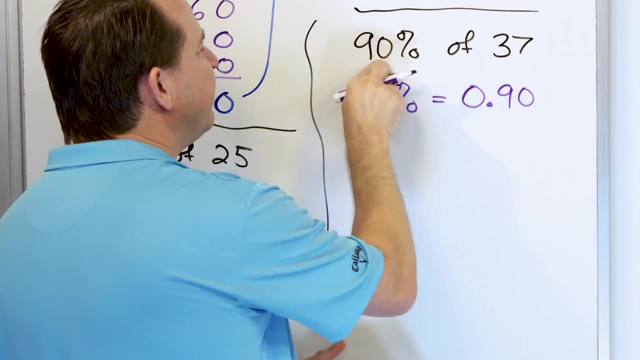 of 37.. First of all, 90% is exactly equal to 0.90, because we can start here and move it two positions to the left: 0.90.. Or you can just say 0.9, because the trailing zero in a decimal after the decimal 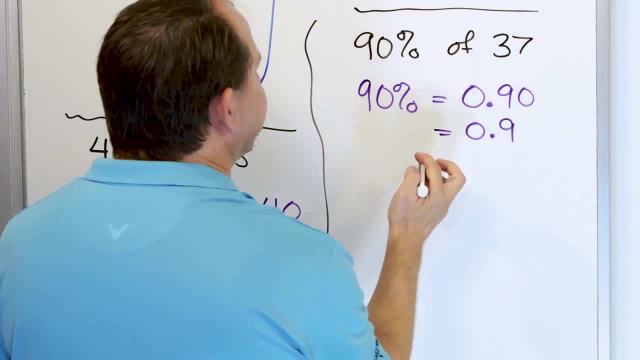 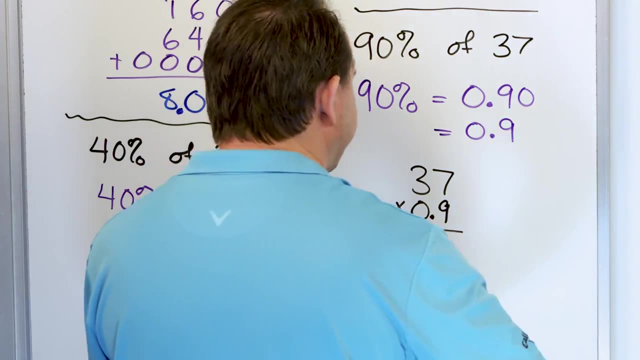 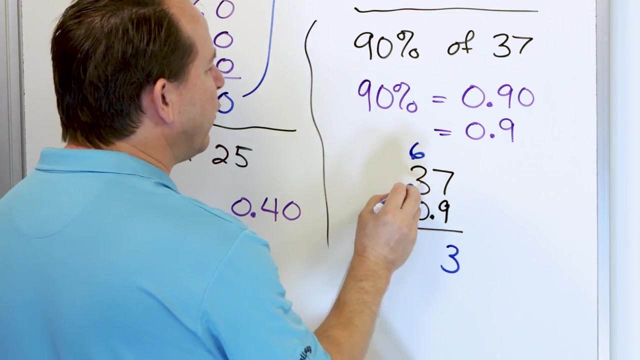 point doesn't really do anything. Then we can multiply by 37. So we'll take 37, 0.9 multiplied like this. All right, Let's crank through it. Let's say nine times seven, 63.. Carry the six Nine times three: 27.. 28,, 29,, 30., 31,, 32,, 33.. 33 drops here And then we're multiplying. 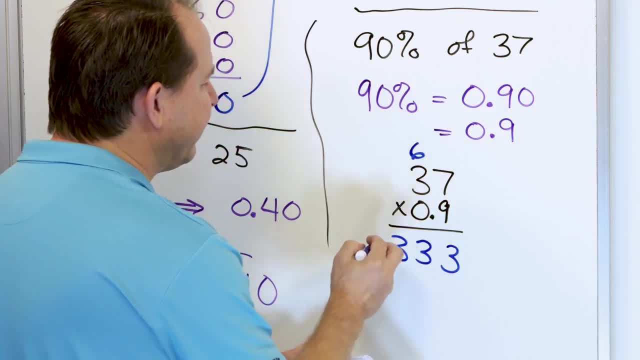 by zero, So we'll drop a zero and then multiply by zero. Nothing will happen, So it's 3,, 3, 3.. That's all we have, And we have only one position beyond the decimal, So we have to have a decimal.